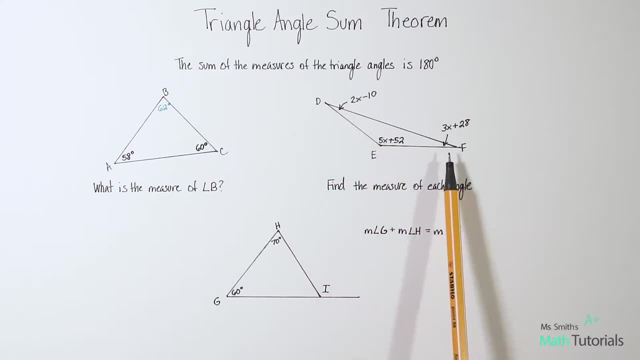 this: I've got triangle DEF And each angle. I don't have any solid numbers like I did in this one right. Each one has its own expression. So I've got triangle DEF And I've got triangle DEF. So I've got to think how could I figure out the measure of each angle? Well, I've got to use that. 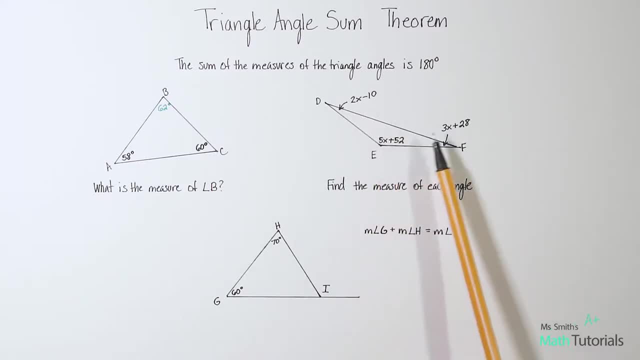 knowledge that I know that these three angles add together to give me 180 degrees. So that's an equation, right there. I want to take my first angle, 2x minus 10,, plus my second angle, 5x plus 52. And order doesn't matter, Meaning I could start here and go here, I could start there, and 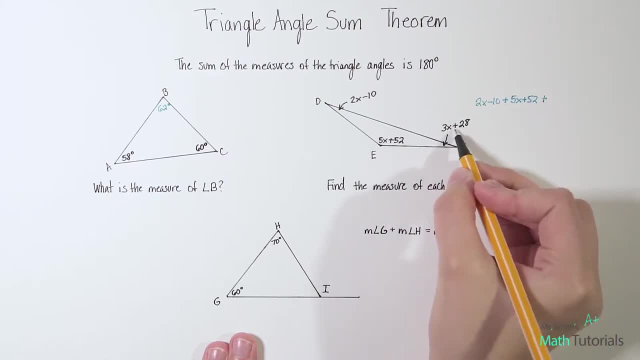 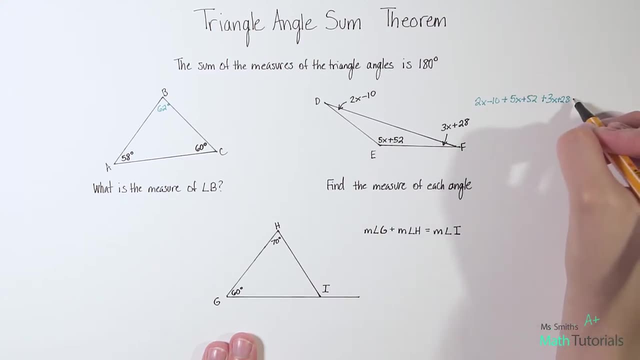 go there, it doesn't matter. plus the third angle, 3x plus 28, and these three angles added together gives me equals 180 degrees. so there's an equation. it's a little long, so I'm going to need to clean it up. I'm definitely going to be looking for like terms here. so I've got 2x plus 5x plus 3x. 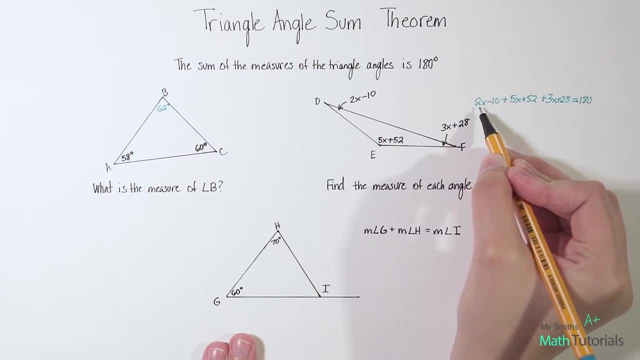 one of 5 plus 3 is 8 plus another 2 is 10x, and then, looking at my constants, I've got negative 10 plus 52 plus 28, so that's going to give me 70. okay, equals 180, all right. we're going to do the same with the other two angles. we've got 5 plus 3 is 1 plus another two is 10x, so that's going to give me 70. okay, equals 180. all right, we're going to do the same with the other two angles. 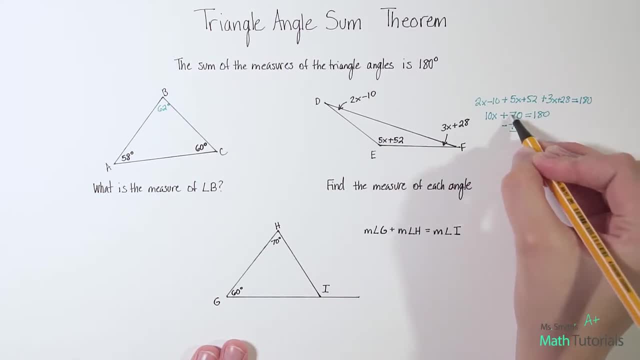 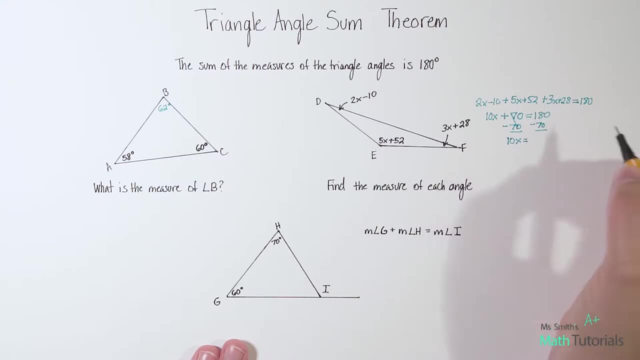 Well, now we're just going to use our inverse operations to solve Subtract 70 from each side. I get 10x equals 180 minus 70.. That's going to give me 110, right Divide by 10, and I get x equals 11.. 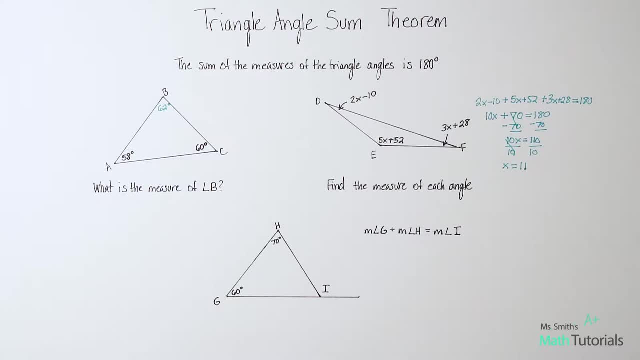 Now I've got to be careful here, because they didn't ask me for x, right? Because we've done some problems in our other most recent videos where they did want us to find the x when adding up some angles, But in this case they specifically asked us find the measure of each angle. 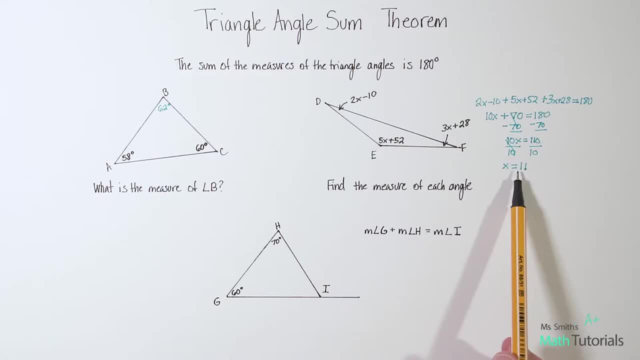 So I've got to take this information of what x is and apply it to each angle to figure out what the angle represents, what it measures. So let's try this one first. So 2 times x minus 10.. Well, I know, x is 11.. 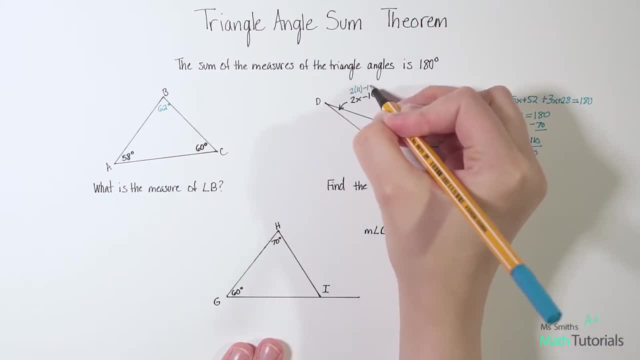 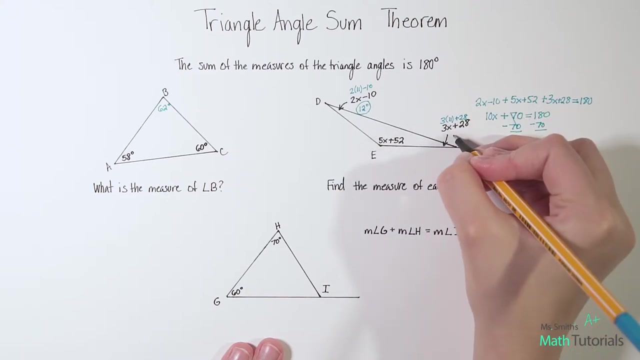 So 2 times 11.. Minus 10.. So I know that angle D is 12.. When I simplify that, it's 12 degrees And angle F, let's see 3 times 11 plus 28.. I know angle F is 61 degrees. 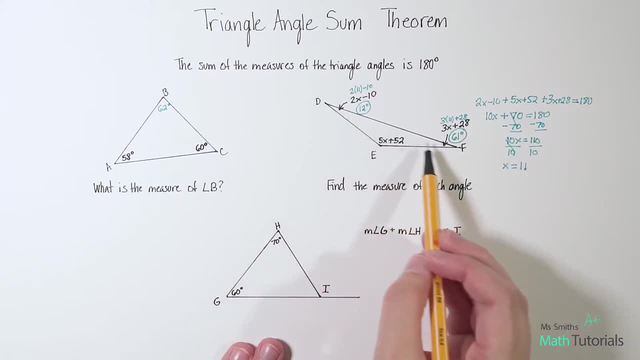 Now, obviously this is not drawn really well to scale because it would not work. It would not make sense for this one to be 12 degrees and this one to be 61 degrees. But I just hand drew these. Just give me some grace. 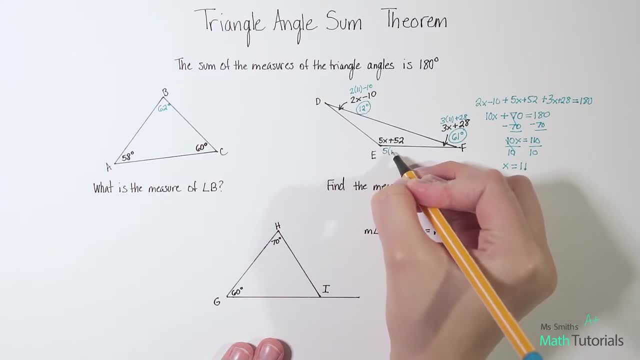 All right. And then for this one, 5 times 11 plus 52. I always try to keep them to scale. So 5 times 11 plus 52. That's going to give me 107 degrees. And then, if you are like me and you want to just double check, 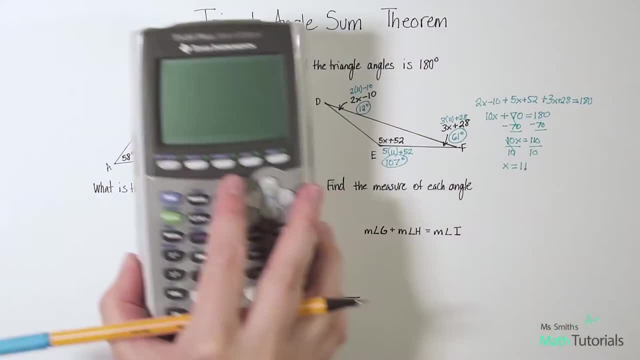 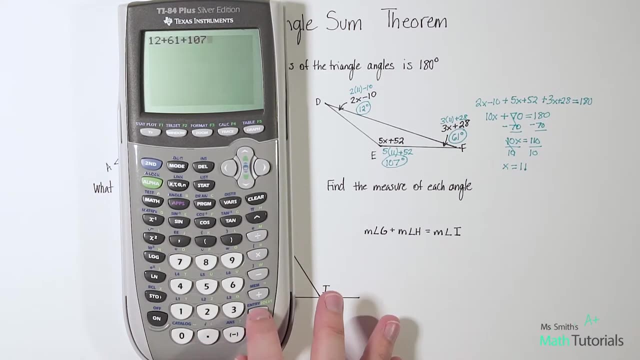 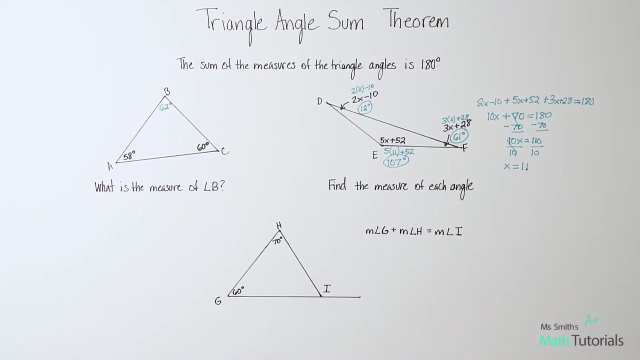 you can just add up all your degrees, So we could do 12 plus 61 plus 107. And we should get 180. And I do So. I can feel confident that I did my math right Now. one thing I do want to talk about down here: 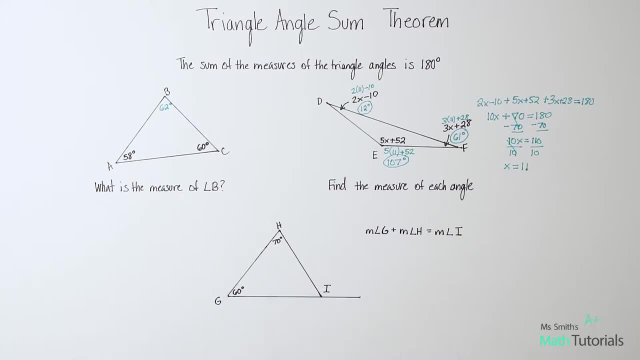 This is an exterior angle rule And it essentially means so. up to this point, with these two examples, we were talking about interior angles, Even though over here I was having to kind of right on the outside. That was just for space, right. 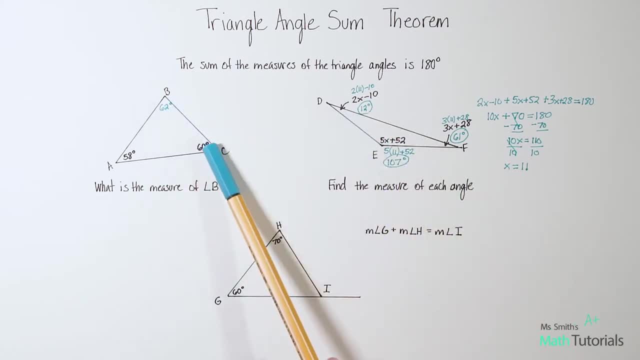 I'm still talking about the inside, inside angles. So we also have a rule for finding a particular exterior angle, And the rule is is that if I were to take this angle and this angle I can figure out, sometimes you'll have, like this, tail right here. 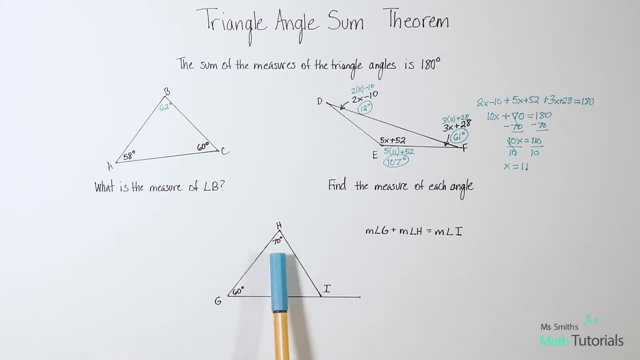 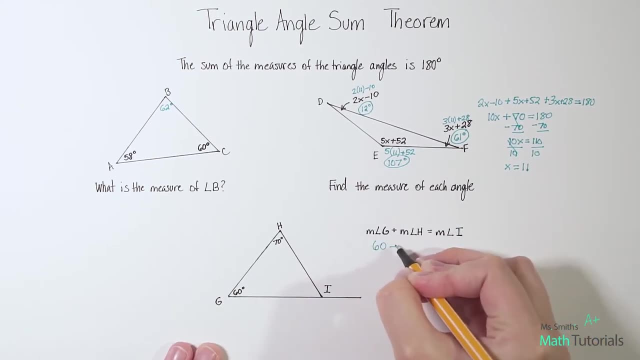 this extension of this angle. Okay, I know that the measure of angle G, 60 degrees, plus the measure of angle H, 70 degrees, gives me the measure of angle I Right. So 60 plus 70, I know is 130.. 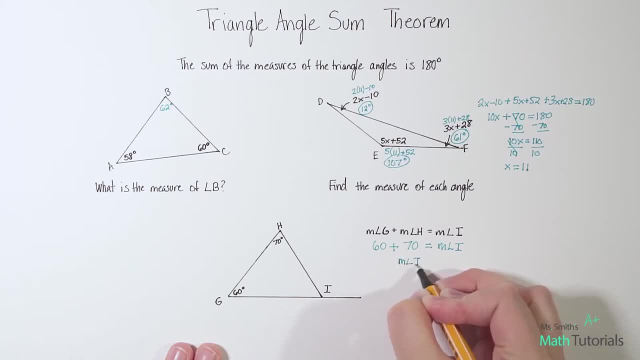 So the measure of angle I is 130 degrees. Okay, So that one's just kind of a little trick. you should know about the exterior extending angle that sometimes, you'll see, I always think of it like a little tail, Like when a triangle has a tail. 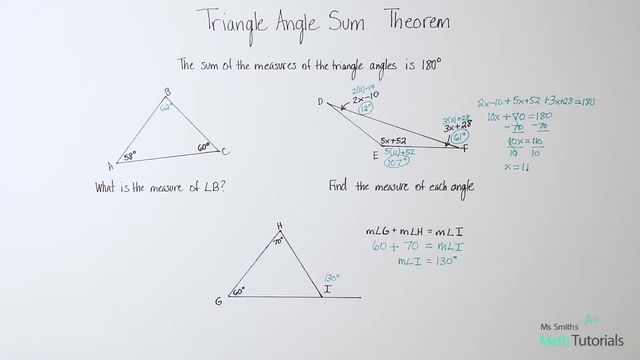 I can figure out that angle by adding up the two on the other side of it. Okay, Not the one right here, not the one connected to it. That would be a linear pair. Okay, These are the other side. Okay, Let's look at a few more examples. 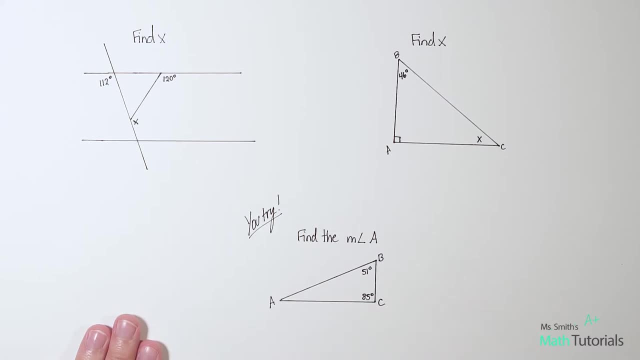 So this one really puts our knowledge both of angles, different type of angle relationships, but also the fact that our triangles add to 180 degrees in action. So I really like this example. They want us to find X, Like what is the measure of X? 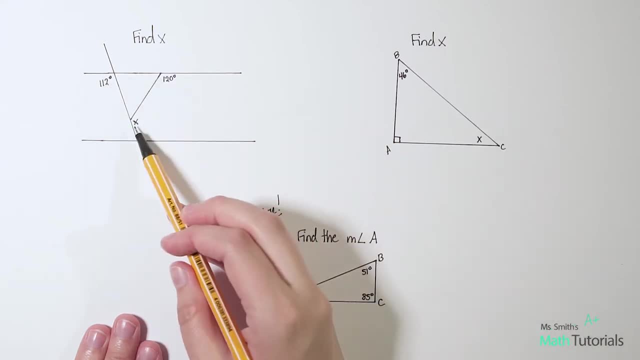 So currently, looking at this, I don't know what X is at this point, I immediately think about starting here. So I noticed that this 112 degrees is a linear pair. Remember I talked about if you could draw like a little rainbow. 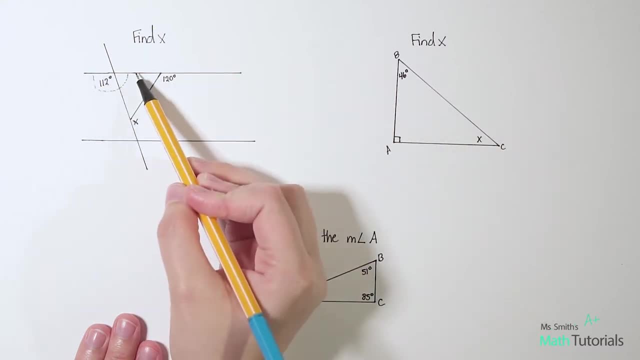 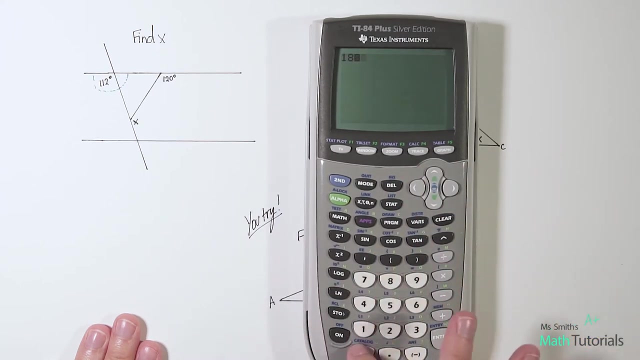 a little half circle, okay, against a straight line. whatever these angles are, I know they add up to 180 degrees. So if I know one of them is 112, I can easily figure out the other one. I just need to go 180 minus 112 and I get 68 degrees. 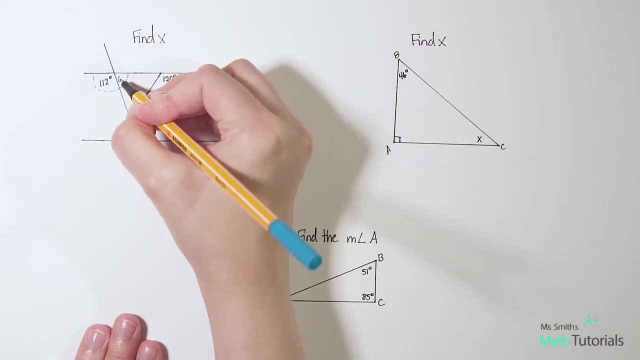 So I figured out what this interior angle is. It's 68. And I can apply that same thinking over here to this 120 to figure out this angle. This is also like a little rainbow, if you will half circle, Okay. 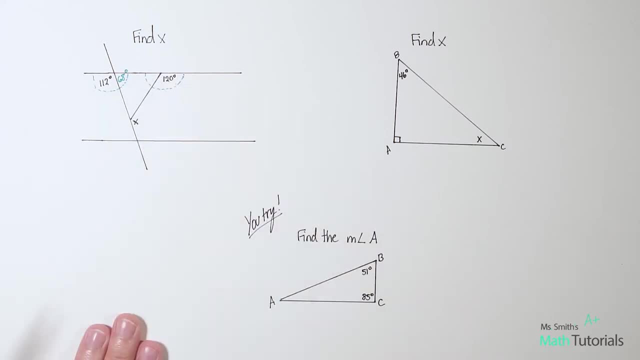 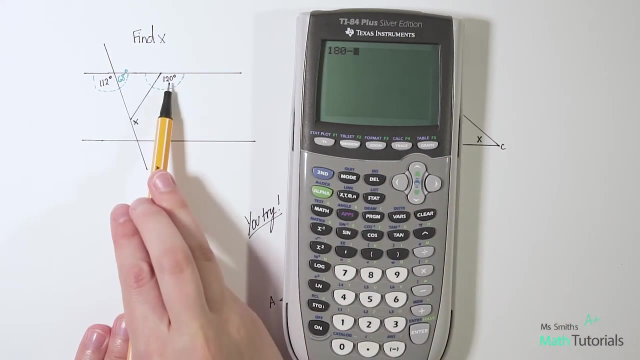 So that tells me that this angle and this angle should add up to 180.. So let's see, if I take 180 and subtract the one I already know, 120, I get the remainder 60. So that tells me this one has to be 60 degrees. 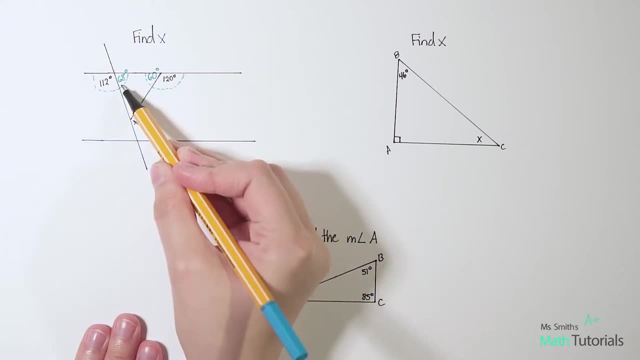 Okay, Now how can I figure out this one down here? Well, if I know, this angle is 68 degrees and this angle is 60 degrees. notice the triangle that's built here, And I know the angles of a triangle add up to 180 degrees. 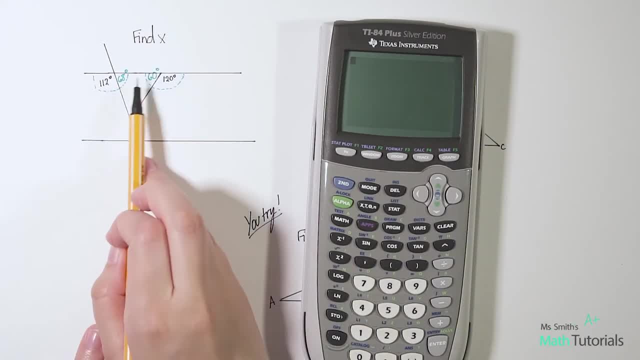 So I want to see what this angle is. What is the? if I added these together, what's my total so far? 68 plus 60.. Okay, So so far those add up to 128.. So now I want to take the total- 180- and subtract what I already know: 128.. 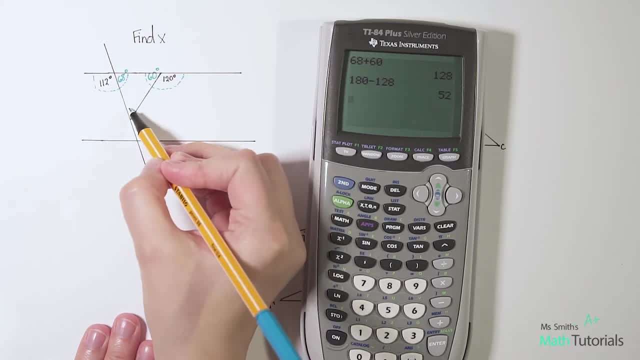 I get a remainder of 52.. So that tells me this angle down here is 52 degrees, And we can always double check ourselves. So I'm going to close out my circles by going 68 plus 60 plus 52.. And I should get 180.. 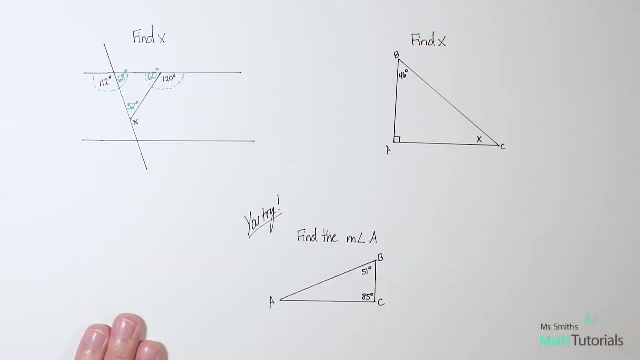 And I do Just as a little double check. Okay, Now, how could I figure out X? Well, here's that half circle rainbow rule. again, If I can build a little rainbow against a straight line, then that tells me that these two- whatever, however many angles are within here. 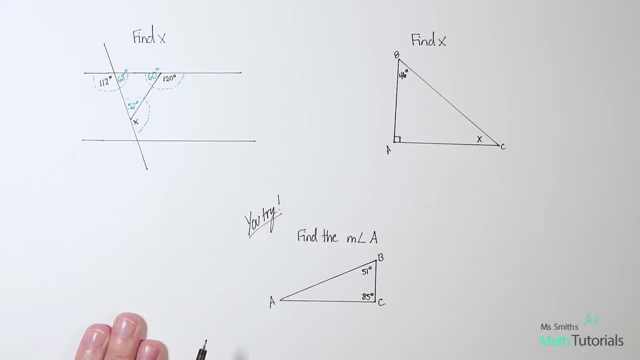 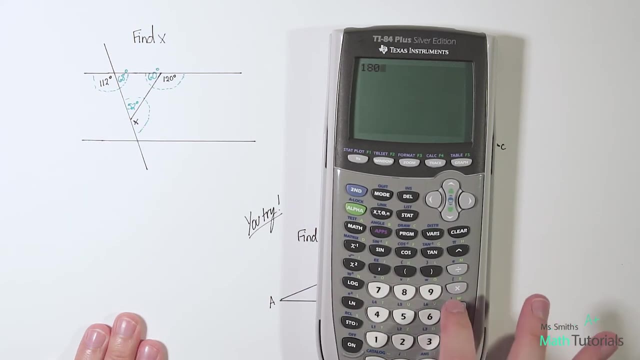 in this case, two. I know they add up to 180. So if I know this one is 52, I just take the total 180, and subtract 52. I get 128.. So now I know what x is. 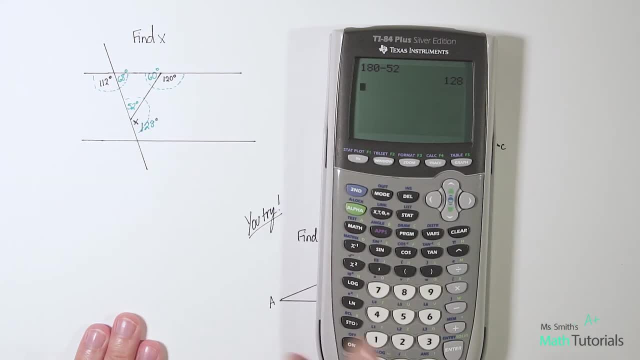 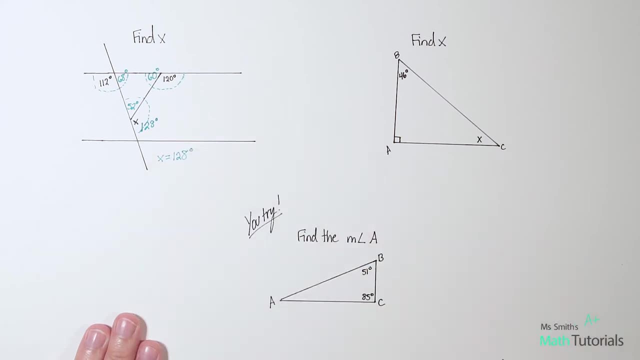 x is 128 degrees. We can write that down here as well: x equals 128 degrees, So I had to do a lot of kind of jumping around to figure it out. Now for this angle, they also want me to find x.